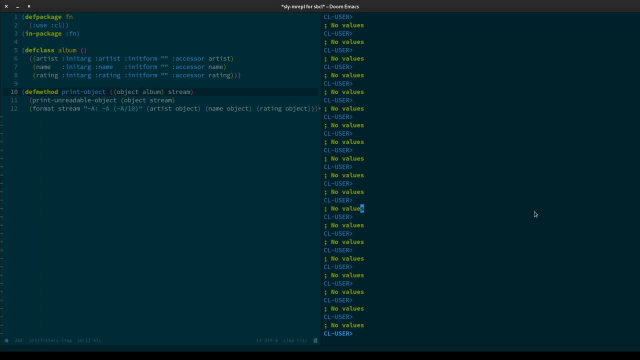 life a little bit more difficult than it ought to have been when I was learning this, because I was applying what I'd learned from Python and JavaScript and Java and other functional languages. So when I was googling for filter, nothing turned up. Turns out, they're not called. 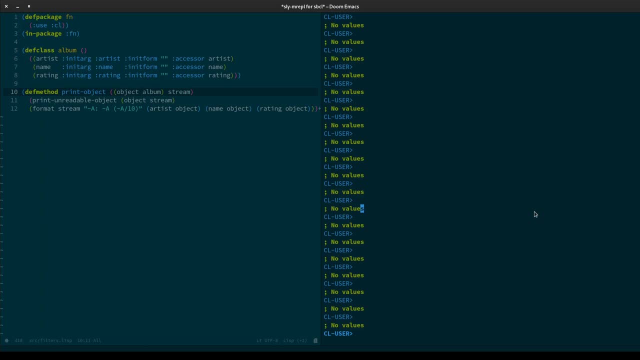 filter in Common Lisp, There's actually six functions that we might want to concern ourselves with, and they are: remove, delete, remove if delete if remove if not, which is deprecated, and delete if not, which is also deprecated. Now, honestly, I don't know what deprecation. 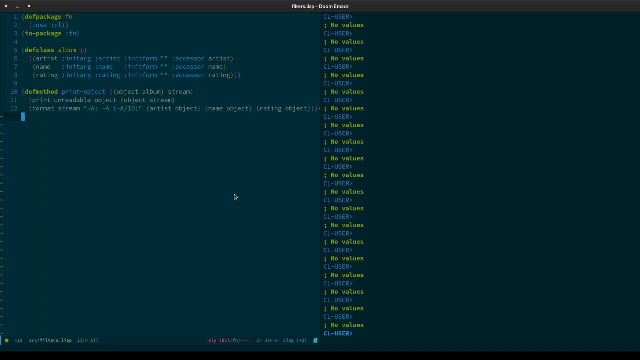 means in the Common Lisp spec since I believe it was standardized in 1994, I think, and hasn't been touched since and isn't likely to be touched again, Because there is enough in the spec to keep the language relevant for decades, like because of the macros and things like that. there's little that you can't later add into the language. 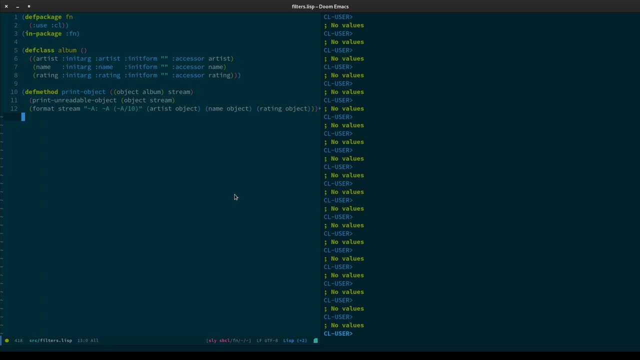 yourself and libraries can fill in for new paradigms and things like that, Which is great, but it does lead to a little bit of confusion when something in the spec is listed as deprecated. Nevertheless, I'm going to cover remove if not and delete if not, very, very briefly, but 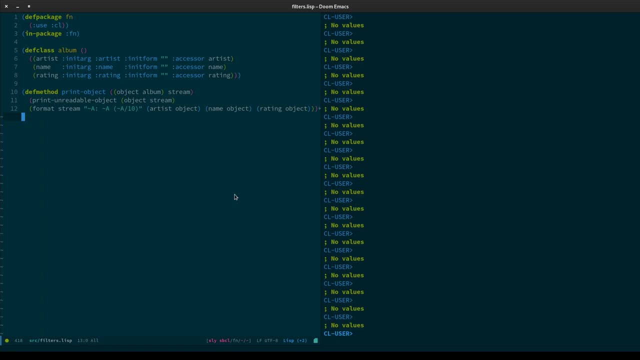 I'm not going to go into too much detail about them. We're just going to focus around remove, delete, remove if and delete if. Now, what you're seeing on the screen here, this is going to help us. This is just a little boilerplate code that I've already, you know, added into. 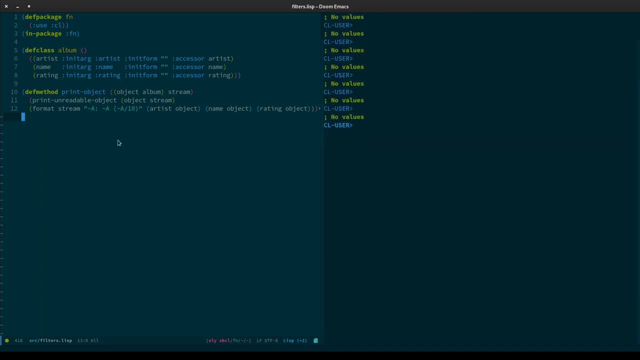 the interpreter, but we'll use that in a little while. We have a few things that we need to discuss, So let's go ahead and remove before we get to that. There we go. So what remove does is: remove takes an object or an item and a sequence and removes that object from the 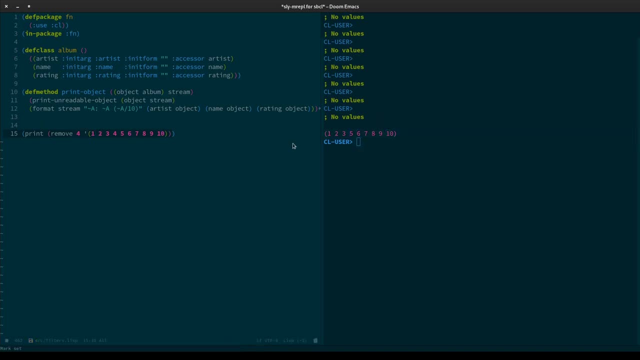 sequence. as we can see here, There is no for in this sequence, So that's pretty cool. However, we might want to remove a slightly more complicated object like a list. As you can see, that list hasn't been removed. The remove function has a keyword argument. 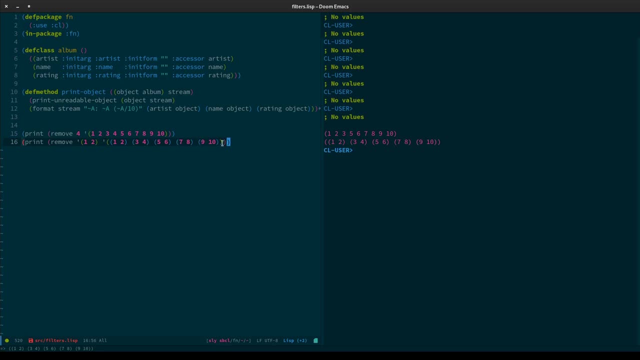 so I'm going to find out whether it is. There we go. I'm gonna say test, There we go The test, if we can hover over here. you can see that the default argument to test here at the bottom of the screen is the eql. 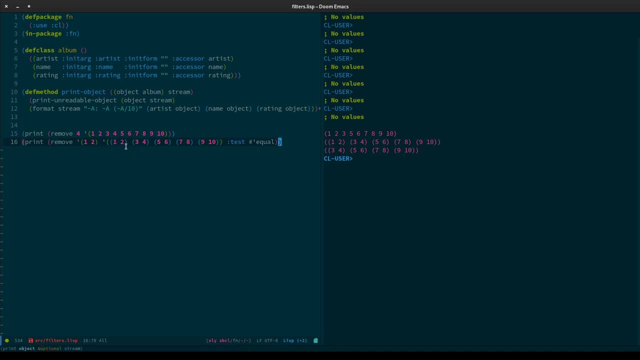 function and that just won't compare lists to one another. So we need to use the test equal function and this will check if that is equal to this list and then it will drop it. So this is how remove works and with the compound objects like a list. so we want to use that test there We can also. there's a 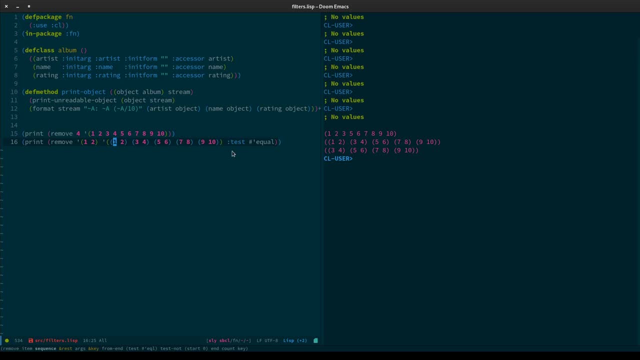 lot more to it. if you look at the bottom of the screen, we've got from end test test, not start- end count and key. So let's have a look at test nots. That's possibly the easiest thing from where we were going. I really shouldn't. 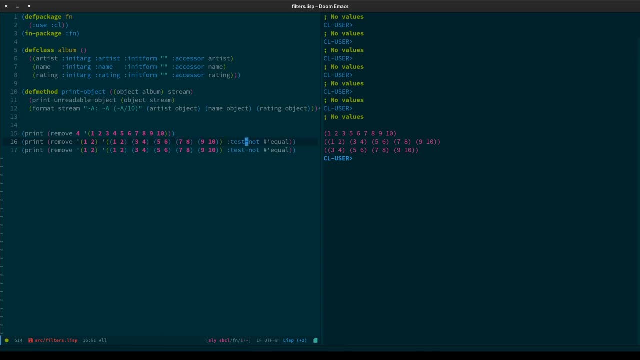 delete the examples. I should just leave those there. So we've got that. This does the inverse. So we're gonna remove, we're gonna modify: remove from the list one and two where they're not equal to one and two. So a little bit counterintuitive, especially if you're used to filter from. 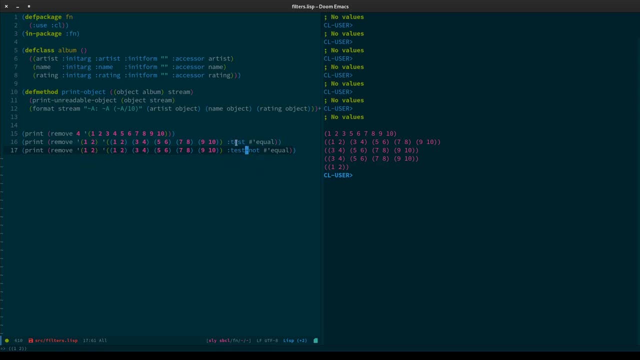 another language. But these tests and tests nots invert the function. so that's what we're looking for in, This is our needle, this is our haystack and this is what we want to do. We're either looking for that or we're either looking. 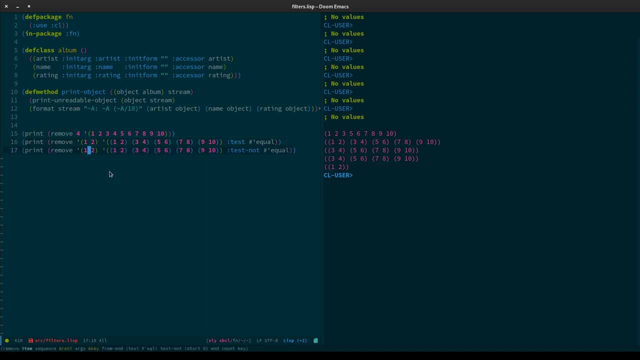 to remove this, or remove everything that is not the needle. So maybe that's better terminology to think of this as needle and haystack and what we're going to do. either we're going to try and lose the needle or lose the haystack. But yeah, that makes sense in my head. So something else we can do. we are going to 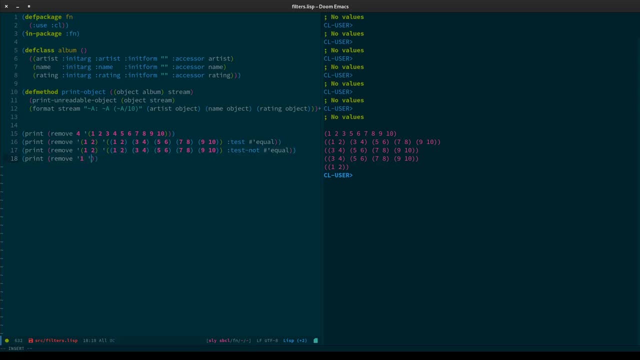 try to remove number 1 from the list of, and what we're going to do is we're going to cast a count. So we are going to remove this needle, this 1, from this haystack of 4, 1s, a, 2 and. 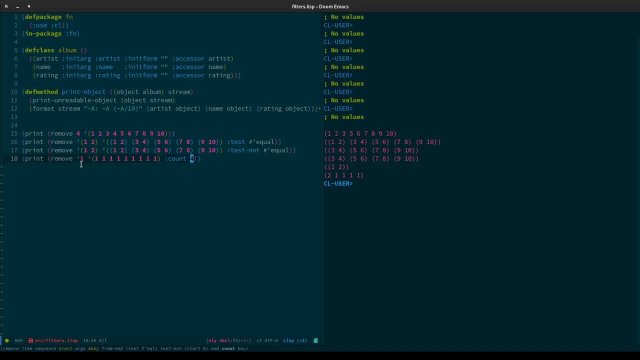 4: 1s to count it four times. So the first four ones get removed from the list and then, from two onwards, we continue because this is zero. one, two, three and four. So we've counted four and two. failed Check because we're trying to remove one. So that's how. 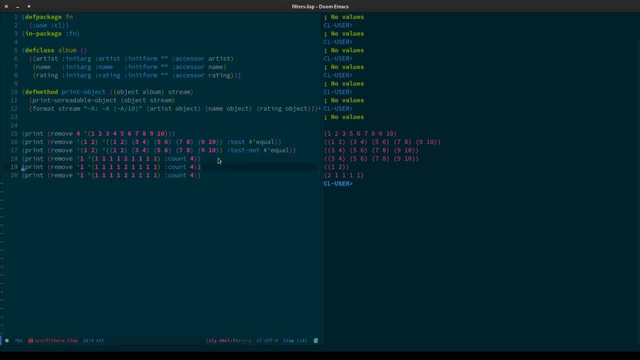 we get that. There's something else you can use if you want. From end: by default is nil, But if we do this we actually start removing the ones from the end of the list to the beginning. But if you omit the count, it is actually exactly the same as just saying. 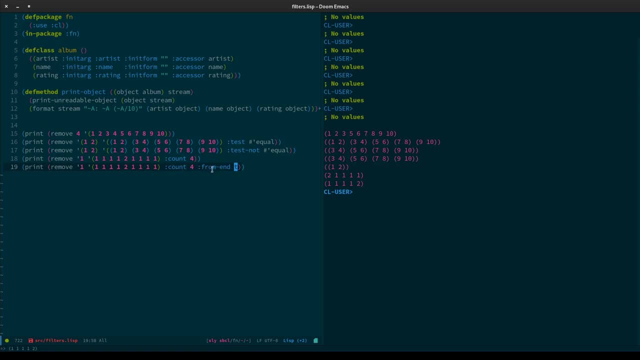 remove one And it might even be slower because it has to go to the end of the list and move forward rather than start from the beginning of the list and move back to the end. So if you're not using a count, there's no point using a from end. It is basically a way of. 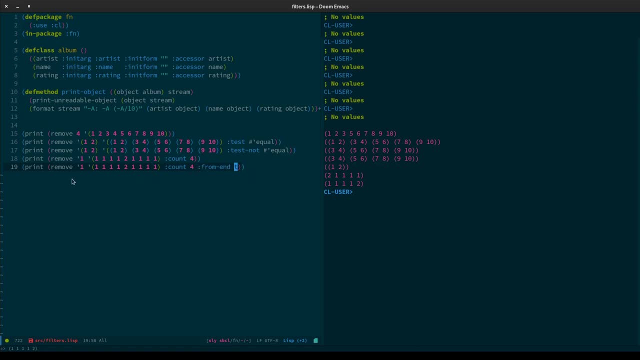 just dropping things from the end of the list up to a certain point, otherwise you just remove them all really. So there's no benefit to using from end without using a count. So that is that We can also do this. We have a start: Get rid of the from end because contrary. 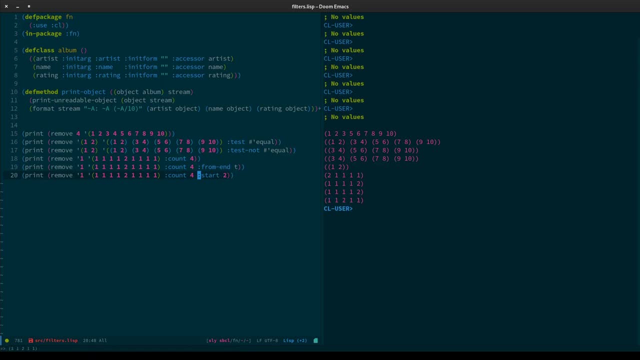 to my advice I have just proven to you. So we're going to start from the second element. So that would be zero one and starting here, And we're going to drop that for four. Then we go here and we drop that, and we drop that and we get these two ones hanging off the. 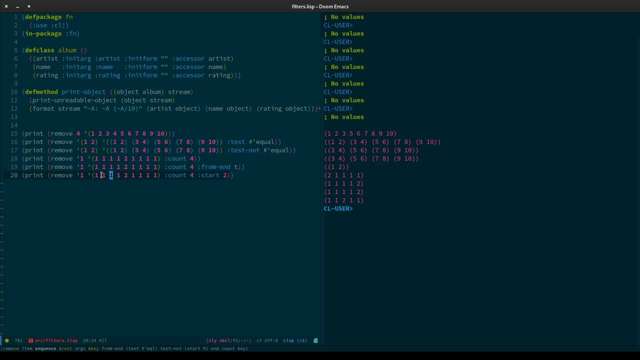 end there. So we've dropped the first four ones from the list that we can find, starting at the second element. So we've got this start thing here, As with the start we can also specify an end. so I'm just going to count 1, 0,, 1,. 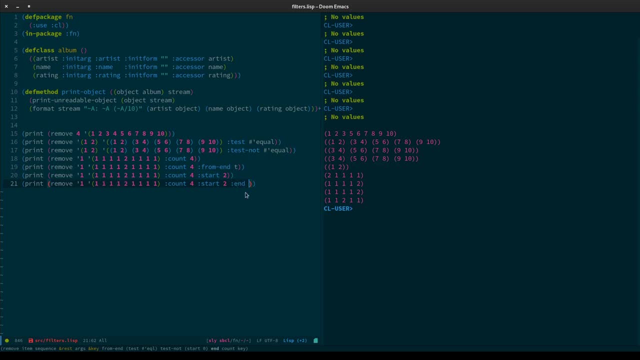 2, 3,, 4, 5, 6.. We're going to stop at 6.. I guess that overrides the count. Did not know how those arguments would interact, so that's interesting. But with the start and the end we can start from the second position, which is here removing 1s. So we'd remove. 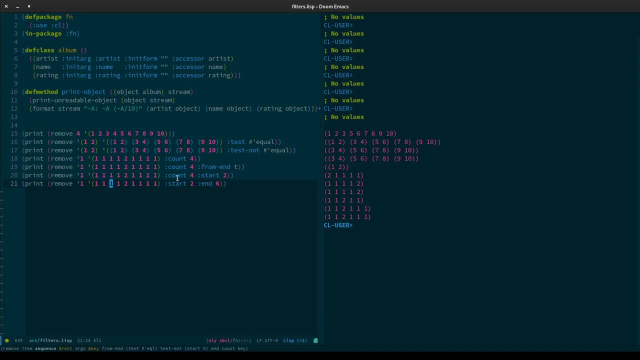 that. so we've got that 1,, 2,, 2, then we stop at the 6th position. So that's where the start and end and we have, I believe, 7 keyword arguments. so we've got 1, 2,, 3,, 4,, 5, 6.. 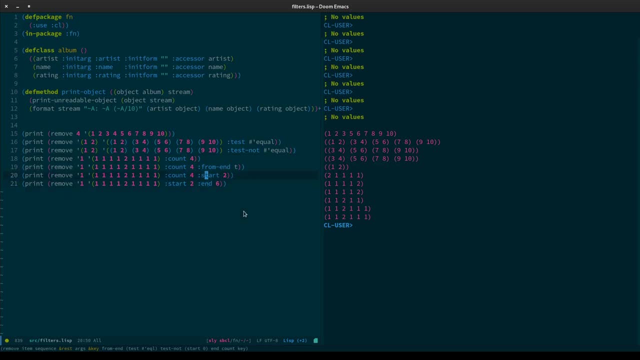 So really, we're only We're looking at this 7th argument now, and this is the most confusing thing, because you have to use it in conjunction with the test. So this is the crazy bit. That's why we've got this code here. This is what we're going to use this for. We're going to create. 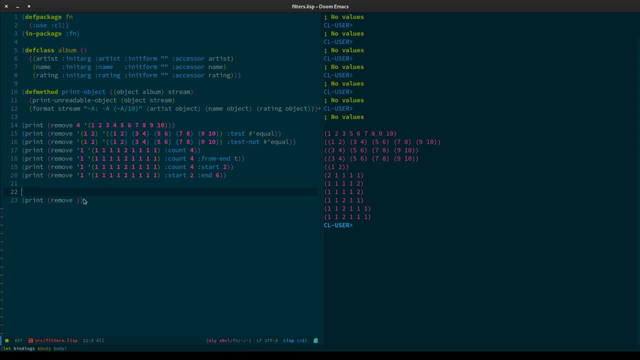 a list of albums and, honestly, I don't know if you've heard of it, but it's a code that looks a bit like this. I'm sorry, this is a very overrated album. in my opinion. It was like mediocre at best. There's some good songs that are pretty good, But if we 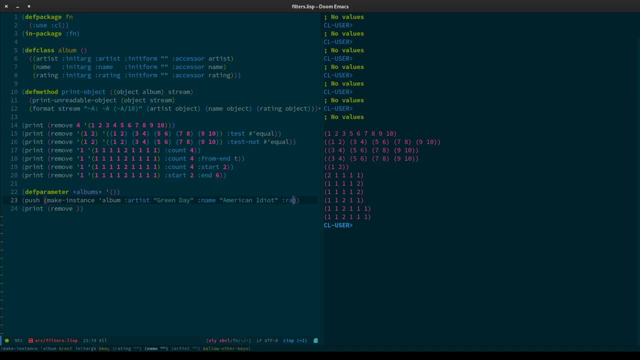 're looking at 4, and our answer here is 5, then we have: well, let's do this. so it's a test here. OK, Good on it, but you know it's not the best album I've ever heard in my life. But you're not. 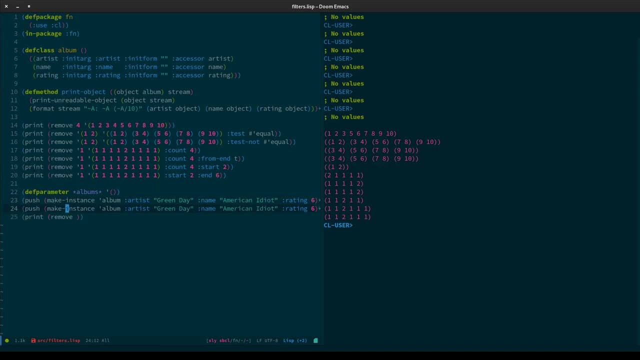 here for my music reviews. so take that with a pinch of salt. If I've offended your musical sensibilities, I am sorry, but we just need test data. That was a good attempt. There we go, so I'm going to evaluate that. I'm going to input this data into the list. 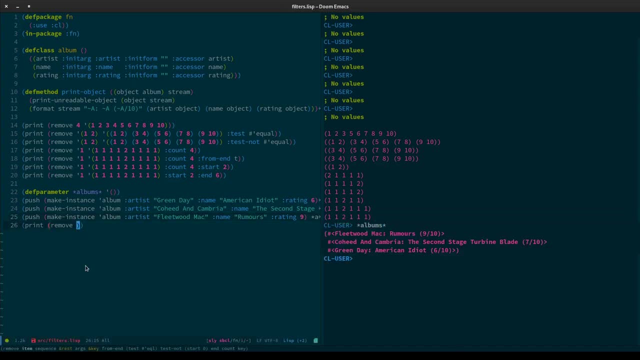 There we go. we've got three albums, So what we're going to do is we're going to remove albums that are seven or less rating, So we're going to remove seven from the list. and we're going to remove seven from the list. So we're going to remove seven from the list. So we're. 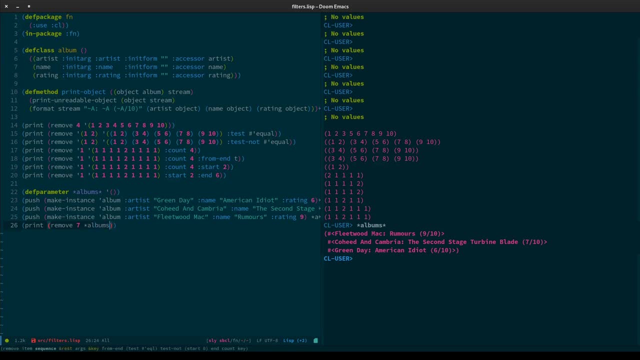 going to remove seven from albums. We're going to test. Oh, that's right. Sorry, There are six or less. This is just an out-by-one error on my part. I apologize, because this is seven. We need to be, you know, six or less, because this basically maps on two. 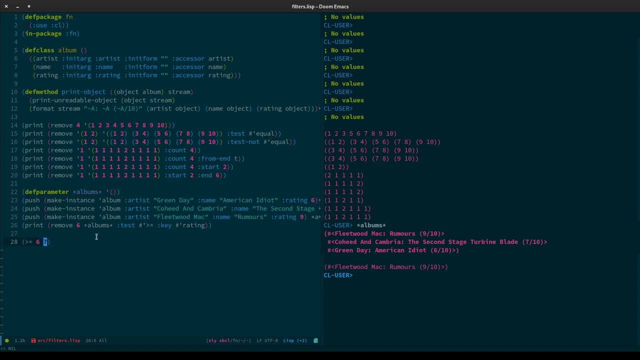 This is false, because this gets passed as the first parameter and that the second, and I always get it the wrong way around just because I'm reading it left to right. I have a bit of a backwards way of thinking, So this will fail, but in reality this is: 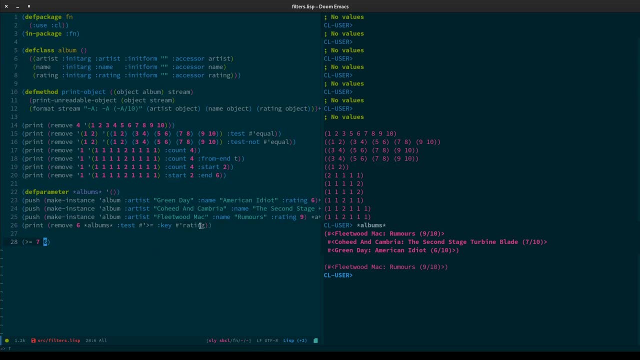 what we want, So that now I have a forwards way of thinking. I'm reading this as the first argument that. So this is how it actually looks. you know, six bigger than seven. So six is the second parameter to our test function. here, Rating is the input. So we're going to 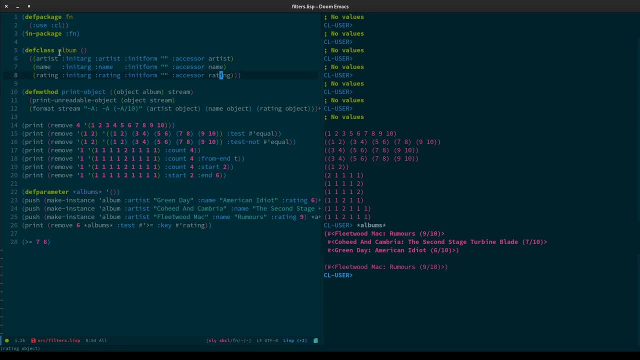 use the implicitly created accessor function method for the album. So you know it's basically the same. as you know, we get nine for the rating of that. So that's what rating does and that's what this test thing. So putting this together, 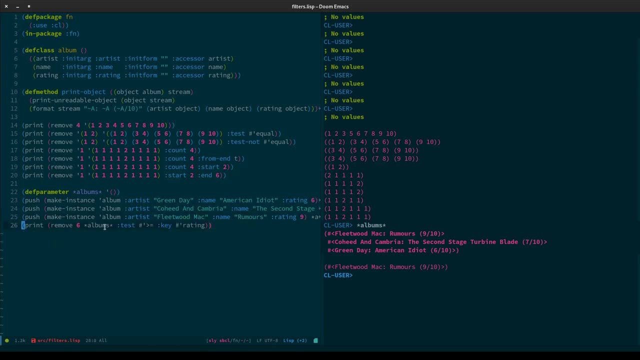 it is the equivalent of saying our test function needs to take two parameters. So we get the first parameter from here and we get the second parameter from calling this function on each item in albums. So this has to be a one argument parameter. This is a two argument. 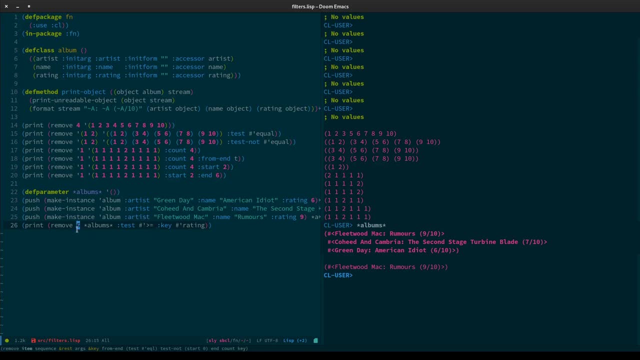 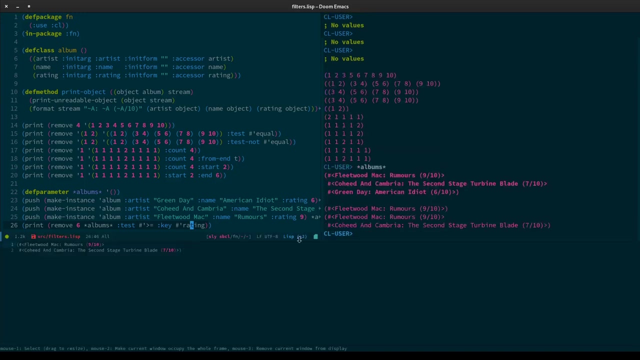 parameter, because it takes the needle that we're looking for and then it uses this key function on each item in the haystack to build up this stuff and return us this. So we'll get rid of that. And we've got Fleetwood Mac and Coheed and Cambria that are bigger than six. 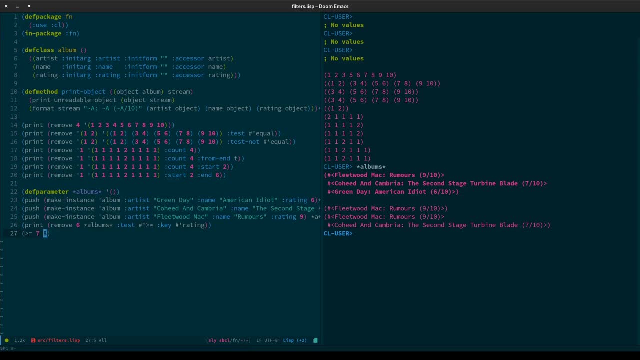 Let me just check. Yes, that returns true. So remove drops items from the haystack that fail this test at the end of the day. So that is pretty cool. That is how you can, and I like the way this looks. This is really, really expressive. It takes a while to get your. 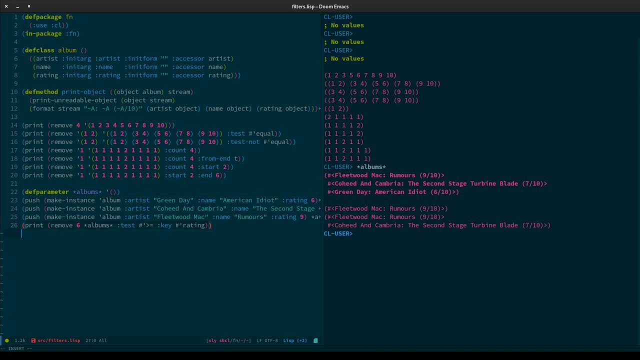 head around it, but it's pretty cool. So we've got Fleetwood Mac and Coheed and Cambria. that are pretty cool. However, this is if you're comparing objects by two things. if you're wanting to do something pretty advanced, If you're just wanting to remove one item that repeats in a list, that's. 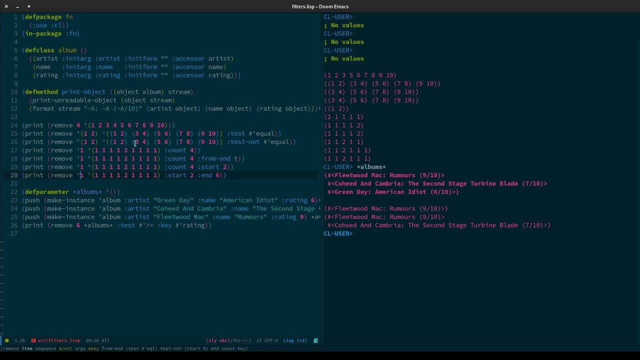 fine, And you can do test for equal, but this will compare the needle to each item in the haystack. So this is a two, So this is a two parameter test and it's two parameters when we're using remove. However, if what we're operating on, if we're just wanting to drop things from a list, 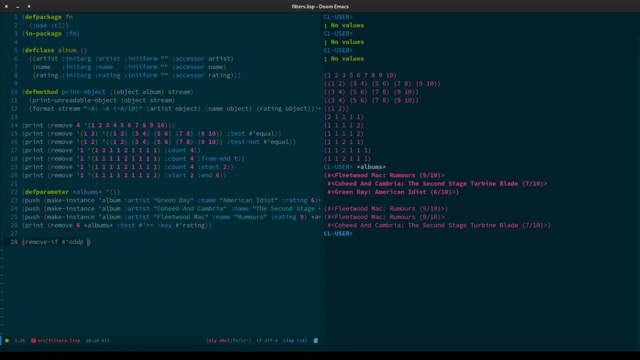 that you really only need one thing, like if you want to drop all odd numbers from a list, We can use remove if, because it's- and it calls it- predicate. yeah, So if we have a look here at remove, you can see that we've got all these extra keyword arguments here. 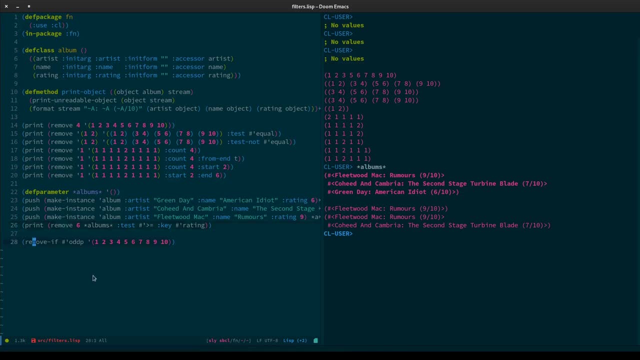 from end test test, not Remove if doesn't have any of that. it just has a single predicate function here And it can take a key, And it absolutely can, and I'm sure I've got notes on that, but maybe not. 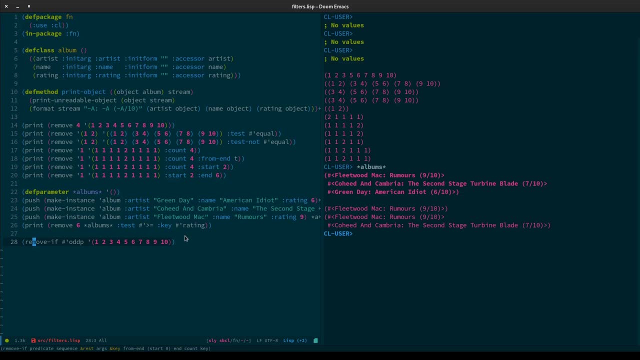 Excuse me while I rifle through them. Yes, we can. So we can express what we did here using remove if, and I'm just going to do that now for you, So we can pass a lambda function in, And this will take one argument, so this will be a rating. 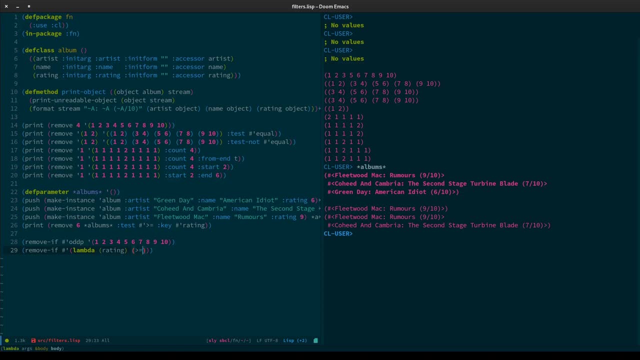 I mean not yet, but it will be, And this is going to be bigger than or equal to six And it's going to take rating And we're going to pass in albums, We're going to pass in the key function and, again, this is going to be rating. 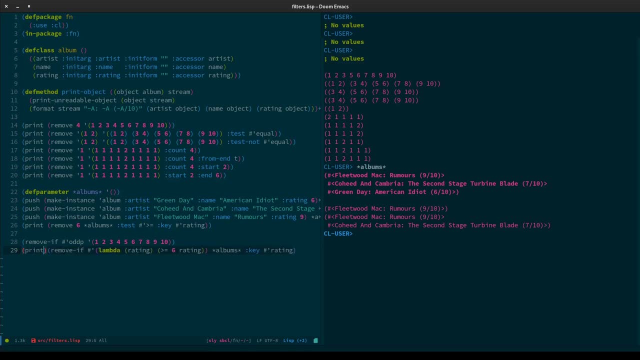 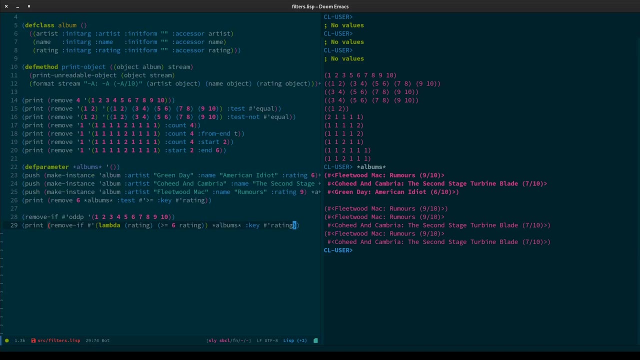 And I'm just going to print that. There we go, And you can see here that this has done exactly the same as that. But we had to write this lambda function that takes a rating and it does all of this And we use the key function again. 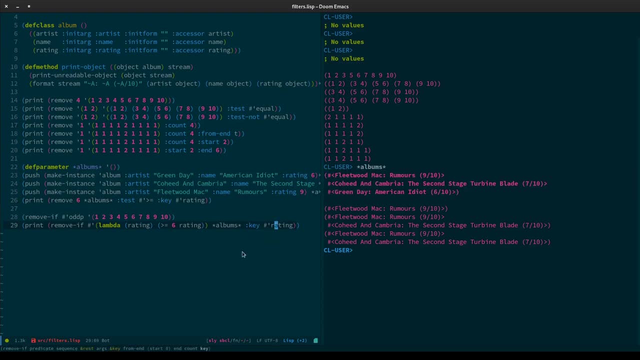 Again to get the one argument function that each of the objects gets passed into. But our function here takes one argument And we hardcode the value in here. So this is how I was used to writing filter functions When I'm working with stuff like this. that's two arguments. 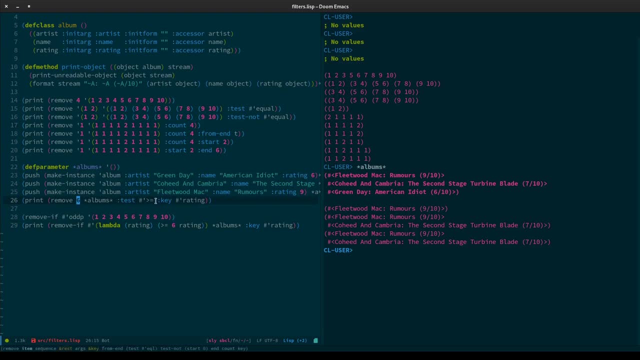 I find Um, Um, I think I would rather use this than this, just because I've already got these functions built in. I'm having to write a lambda function around built-in functionality to the language And looking at this in the function, it's kind of like a magic number. 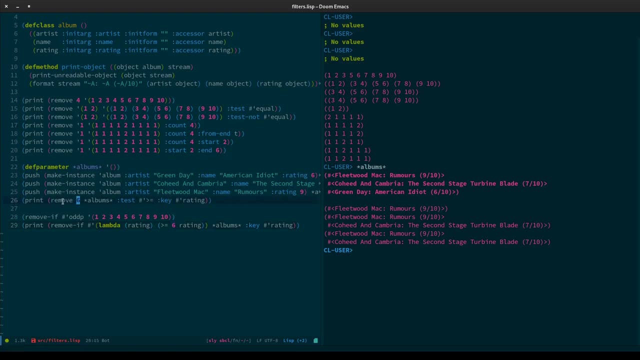 You don't know what it is. We're removing six here. That's pretty obvious based on the test and the rating. Here, in the middle of a lambda function, it's probably less obvious. So the way I'm choosing to view it is. I'll put a print here. 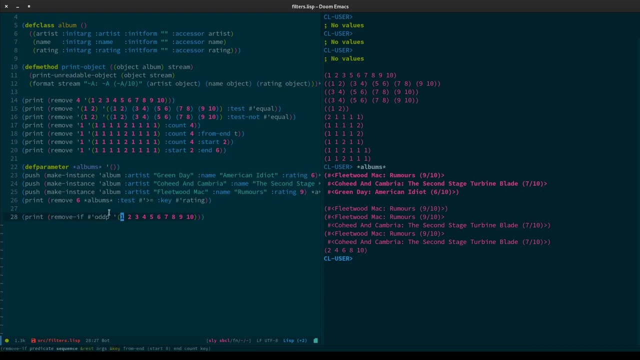 If you are dealing with simply matching a single function to an object in the list, use, remove if, because we can simply make it match a certain criteria- odd, p, even dp- You could have a prime function somewhere that takes a number and figures out if it's prime or whatever you want really. 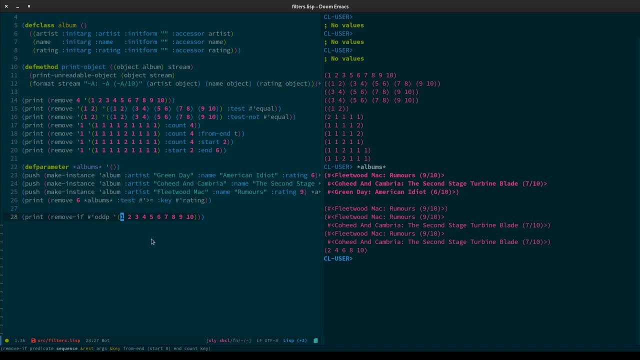 If it's a happy number or even a happy prime, I don't think the language particularly cares. You need a lot of memory for that, I imagine. but hey, whatever. So if it's just a single function that does one thing to an argument, I think the remove if is the most important thing. 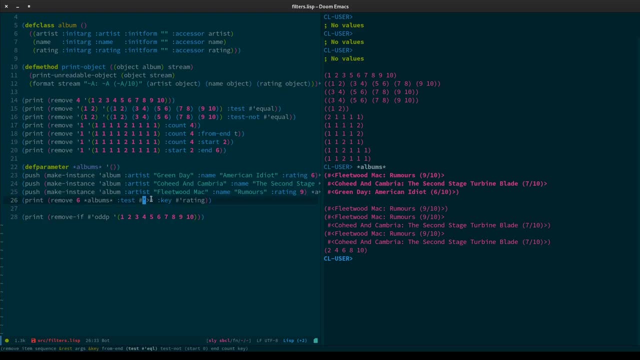 That's the way to go, But if you're doing sort of complex operations where you need to compare one thing to another using keys, the remove form looks nicer to me. Now, for completeness sake, this is our remove. if odd p Our remove not is the inversion. 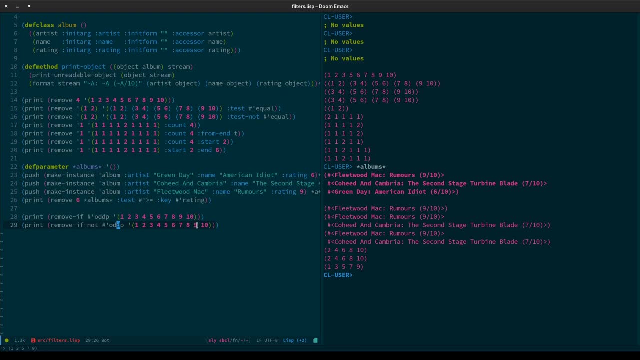 So you know, you can do this, You can move this. We always do. No, I don't think it would be possible to use a. I really don't think this is going to work. Yeah, no, No, that absolutely does not work and I wouldn't expect it to. 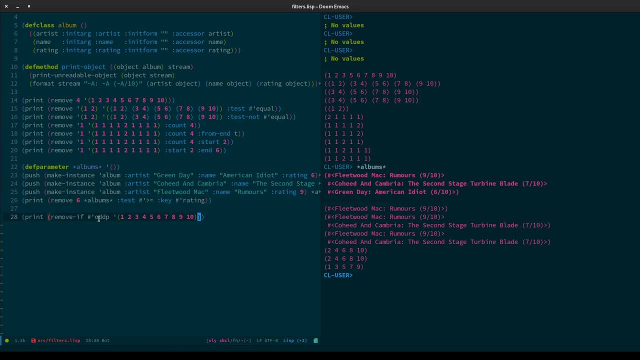 I was just curious. So what we could do here is: if this was Yeah, no, No, that absolutely does not work And I wouldn't expect it to. if this was odd p, we could simply do even p. but for a more complex example again, we could do: 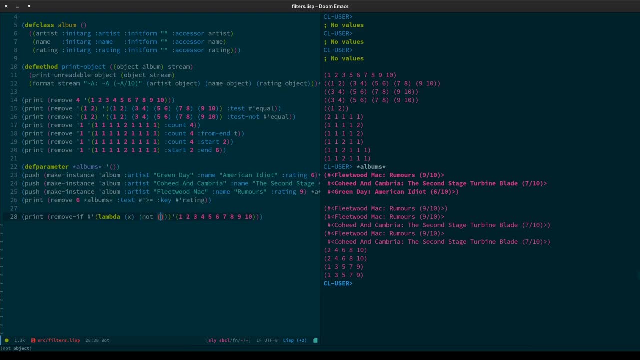 lambda x, not odd p x, and we would get the inverse of whatever that function is doing. we could build up using a lambda function. so i see why they're saying remove if is deprecated, because everything you can do with remove if not, you can do by writing a lambda function and using, not on your predicate. 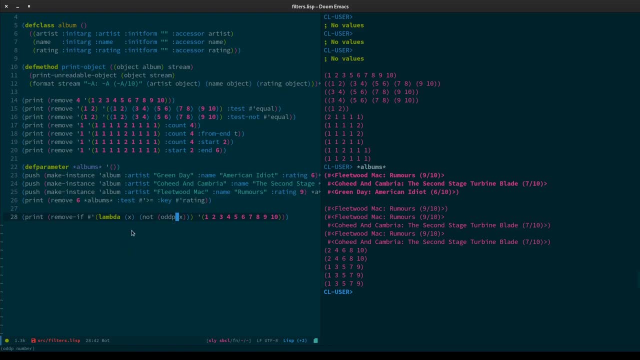 which is probably how it works under the hood maybe, and it's the same with remove- if it's complicated, just just use remove. so that's it for the remove, remove if and remove if not. i'm just going to put these back you, just so that we can see it. for, for completeness sake, 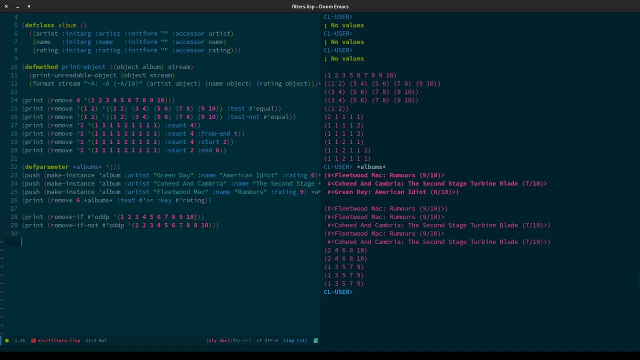 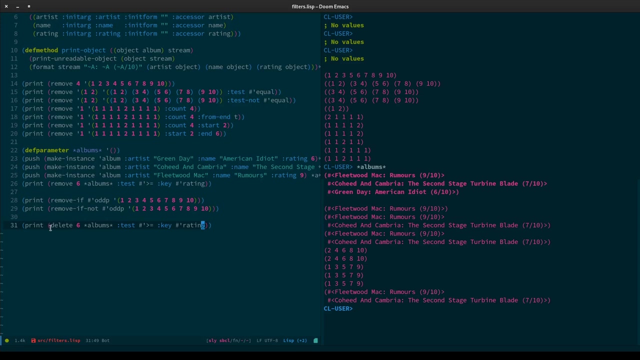 uh, the other thing to be aware of is, um, the delete, delete and delete. if not so, delete is exactly the same form as remove. there's nothing different about it at all except the function argument name, and we got these two things back, um, so we are just simply dropping green day from there. however, 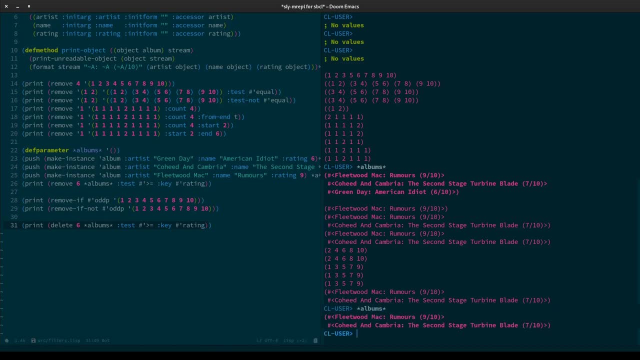 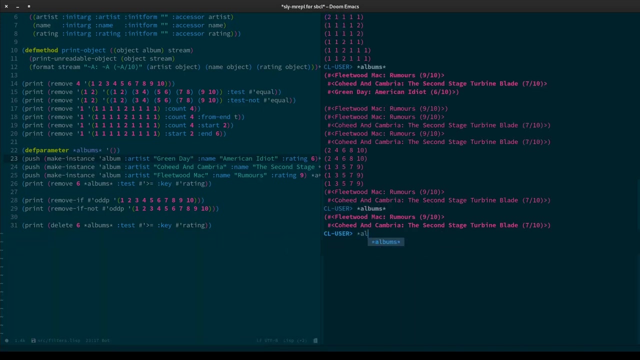 the problem is: delete may alter the original array. so by doing that our albums array has been transformed. so i have to then put this back in and we'll say albums and we've got the three back there again. so if we do that we get nothing. so i'll just put a click here on this um, and i will of course want to say um, but there's three items in there, so it's the spec says that delete. 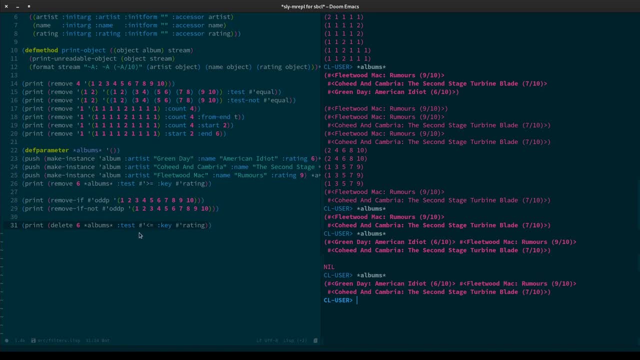 me alter the original list. so it might, it might not its undefined behavior, i believe. so different common list interpretate interpreters might do it different ways. I have had mixed results with it where sometimes it would alter my list and sometimes it wouldn't. so I guess it would depend on the particular. 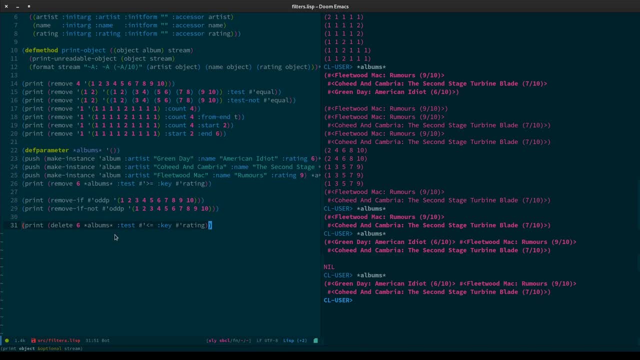 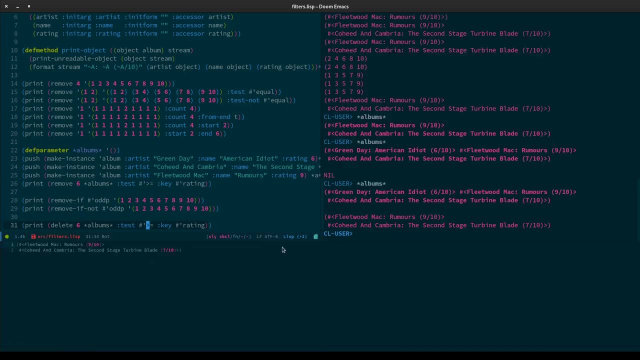 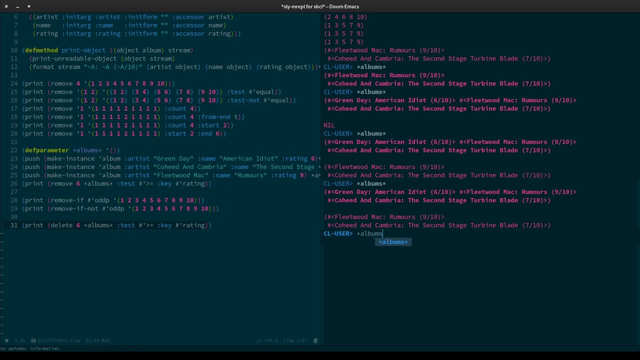 documentation of your interpreter. put that back. yeah, we've got, you know, the three things there and we've got the two now, but yet the three remain in albums. so you know, it can- it can vary. so, yeah, we've got American Idiot come back, oh, and. 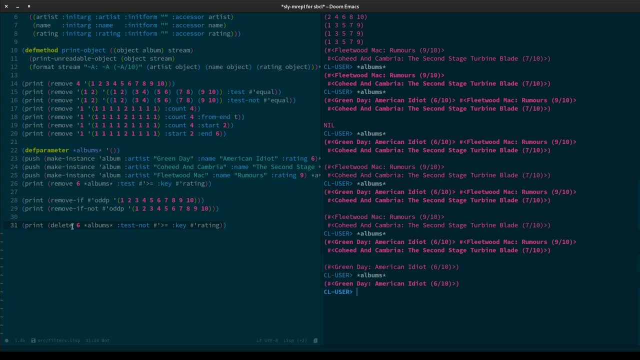 and it's that. so just be aware, with delete, it may not always do quite what you think it does. so you have been warned, whoops. so say delete if- and we're gonna say so- we're just going to evaluate that in. so evaluate that we're deleting. if odd P numbers, we get two, four, six, eight, ten. 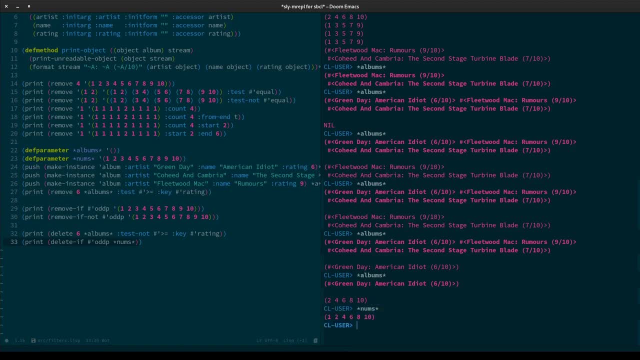 which is exactly what we might expect. however, nuns has been transformed, but one still stays in the list, so that's a bit weird. but__d problems there. delete if returned what we want to. it just screwed up the the nuns. so if we evaluate that again we evaluate it- we get one, three, five, seven, nine. two, three needed four and two, two, three, seven, nine. so we got one, three. 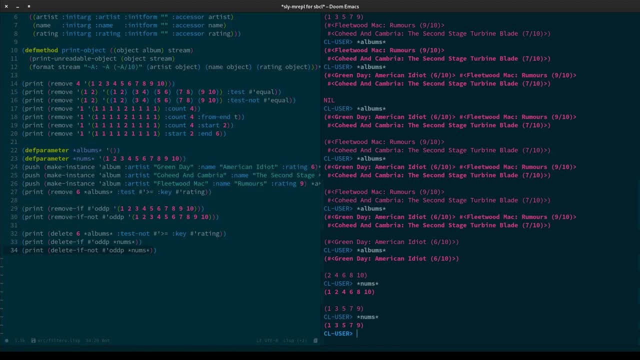 get one three, five, seven, nine, and if we evaluate nums now, having done that, we get one three, five, seven, nine, which is probably what we would expect. so your mileage may vary. if there is a pattern to what delete is doing- I have not noticed it yet, so apologies about that- there might not even be a pattern. I 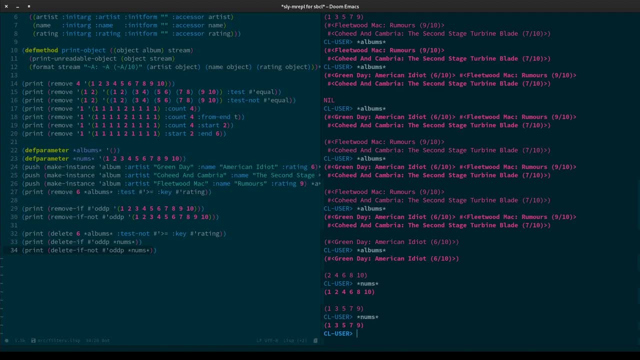 don't know, I'm not again. if there is one, I haven't found it, but this is: you know your, remove, your remove if. remove if not, delete, delete if and delete if not. I tend to favor remove and remove if again, remove if not and delete if not are. 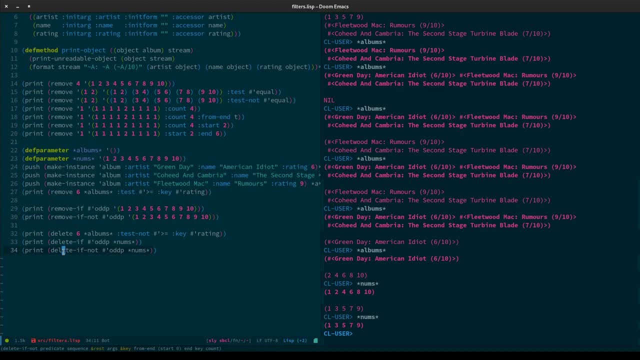 deprecated, although, again, what that means, who knows? so this is hopefully everything you could possibly want to know about filter functions and predicates and common Lisp. next week we are going to have a look at the reduce function and following that we're going to have a look at the map reduce. 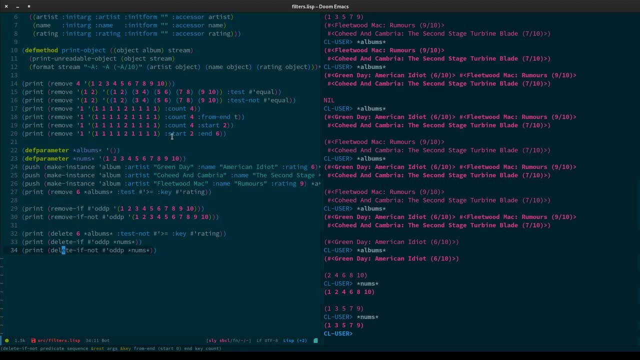 algorithm, which hopefully will be a lot of fun. I hope that was interesting to you. I hope you're enjoying your Friday. I hope you enjoy your weekend and thank you for the massive amount of support my channel received last weekend. it was incredible. thank you. everyone that watched and subscribed liked the videos. 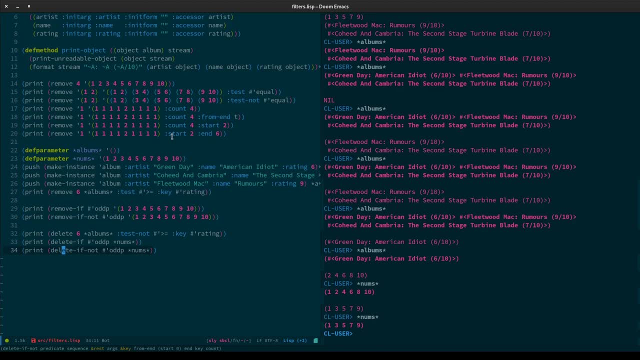 it was a massive help. I don't like doing the please like, share and subscribe thing, so you know. I just want to say thank you for those that that feel they want to do that. I'm not doing it to become particularly famous or anything like that. this is information I've started recording for friends. I've just 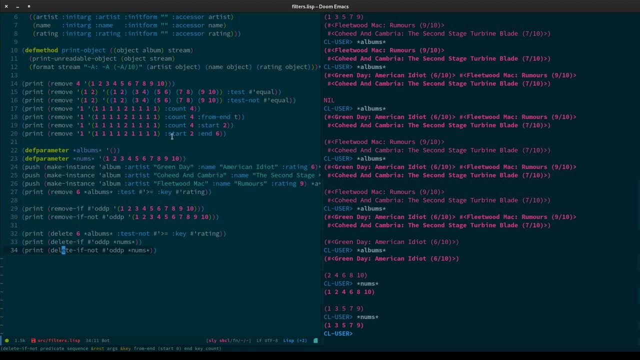 learnt. there is a huge demand for videos like this, so I'll keep making them if you keep wanting me to and as long as I am able to. so again, thank you everyone. take care, enjoy your weekend.